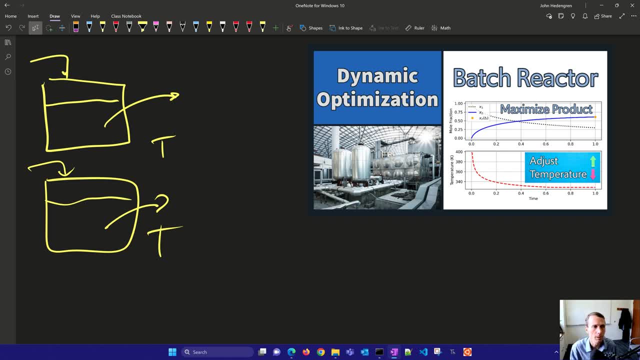 where you have maybe smaller high value production processes, especially like chemical and pharmaceutical manufacture, biofuel production, food and beverage industries and also agricultural production. So these batch reactors, we're going to try to optimize this one where we're going to modify the temperature over this particular time window and try to maximize this product. two in: 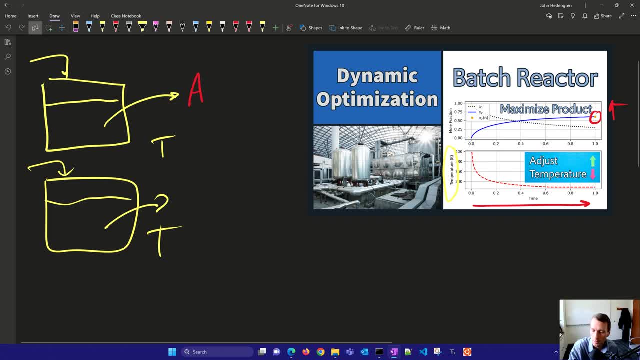 the reactor. So we have a reaction. I'll just say A goes to B, goes to C and the desirable reaction is: A goes to B, goes to C. So we have a reaction. I'll just say A goes to B, goes to C and the desirable reaction is: A goes to B, goes to C. 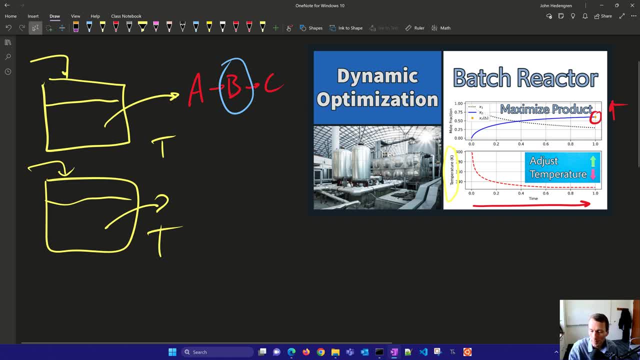 One that we want is going to be this B, and the reactants are A at the beginning and the undesirable one is C here at the end. So we want to try to get as much of this B reactant as possible. Now we've got some equations that relate, that basically help us describe the optimization. 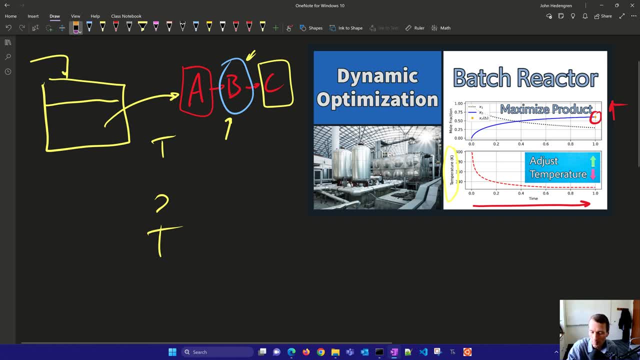 problem and I'm just going to erase some of this here so I can write my equations. okay, so we have some reaction rates that we're going to be tracking. well, first of all, try to maximize- and we're going to maximize- x2 at time final, and we're going to do that by adjusting. 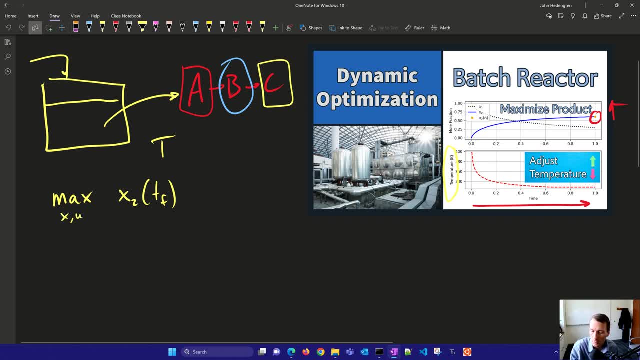 our x and u values. now, u is going to be equal to the temperature. that's going to be our input for this system, and we have a differential equation: dx1- dt equals. and then we're going to have minus, reaction rate one and reaction rate one is right here. reaction rate one is going to 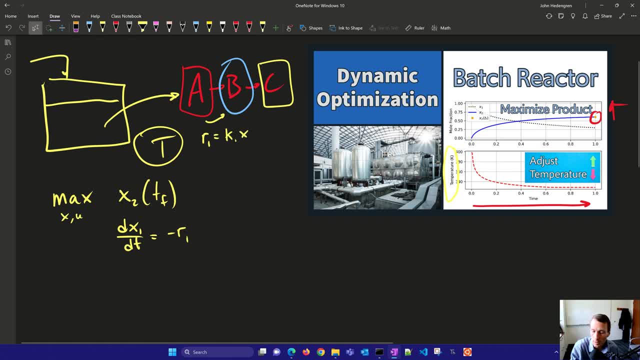 be equal to k1 times x1 squared. so we have this first one. this is a is going to be one. that's our concentration. first one concentration, second concentration, third concentration. so it depends on the concentration of a squared. now let's go ahead and write our equation for the. 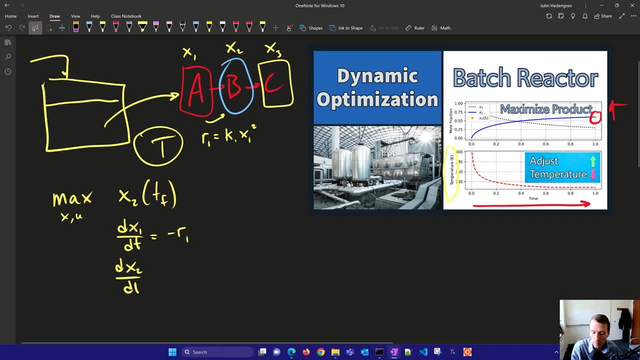 next one, so DX 2 DT. this is going to be for B, and that's going to be equal to reaction 1 minus reaction 2. okay, so reaction 2 is going to be this one, right here, where reaction 2 is going to be equal to K 2, that's just going to be. 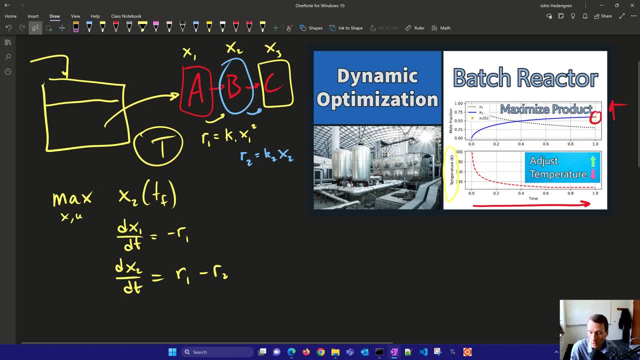 another constant times X 2. so that's a first-order reaction and it's going to control the rate at which B goes to C. alright, and then our third differential equation is going to be DX 3, DT equals, and that's going to be equal to reaction. 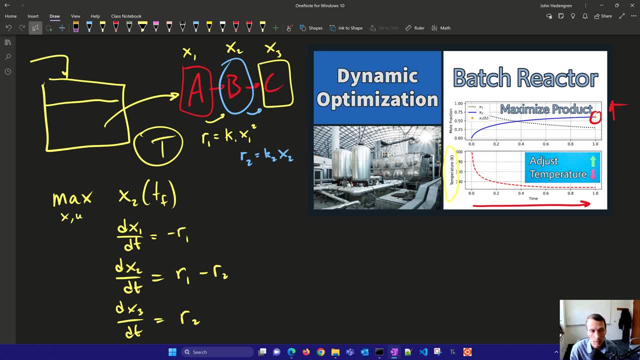 2, so it's not going to be how much is produced, the rate of what X 3 is produced. now, the one we're trying to do is we're trying to do, is we're trying to do. is we're trying to try to do, is we're trying to do, is we're trying to do, is we're trying to do. 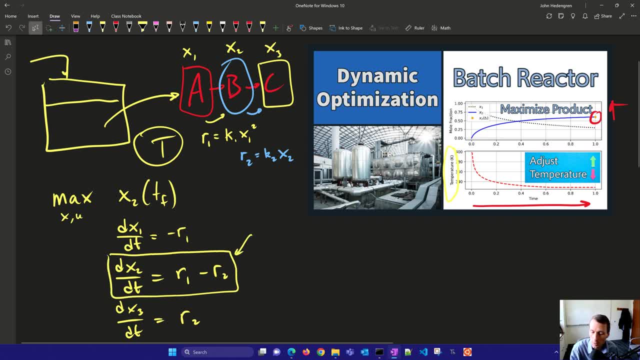 maximize is this one, but you see we start to lose it as we start producing more X 2, so we want to try to optimize this. we've got a couple rate expressions here and I'll just write these out as well. K 1 is going to be equal to 4000. 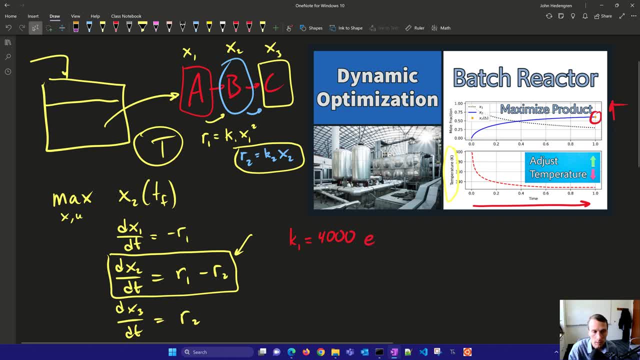 okay, that's our pre exponential factor: e to the minus 2500 divided by T, and here- and I'll just write these out as well- K 1 is going to be equal to 6000. here, and I'll just write these out as well- K 1 is going to be equal to 6000. 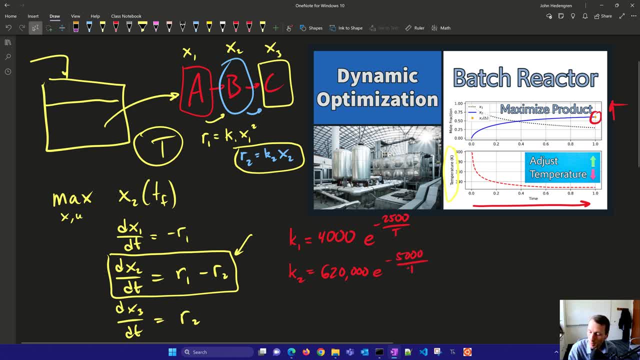 E to the minus 5000 divided by T. so you could see here, depending on the temperature as we move it up or down, we're going to increase or decrease these rates. so I preferentially produce B and not produce as much of this rate C. now we're going to start with an initial condition. x1 initial is going to: 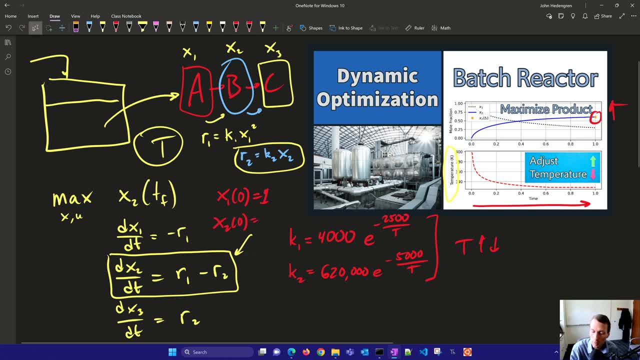 be equal to 1, and then x2, initial is going to be equal to 0, as well as x3. okay, all those are going to be equal to 0. now I can go somewhere between temperature of 398 to 298. okay, so plus or minus 50 degrees in there a hundred. 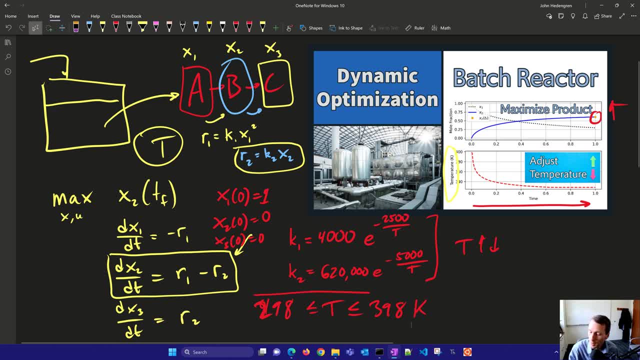 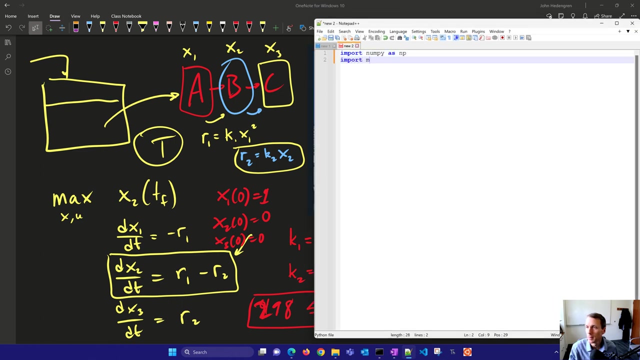 degree range, total and Kelvin. okay, so that's my manipulated variable, the thing that I can adjust in order to try to maximize x2 at the final time. so let's go and just write out the equations for this and solve it with Geckos go. so, first of all, going to import numpy as NP and then I'll import map. 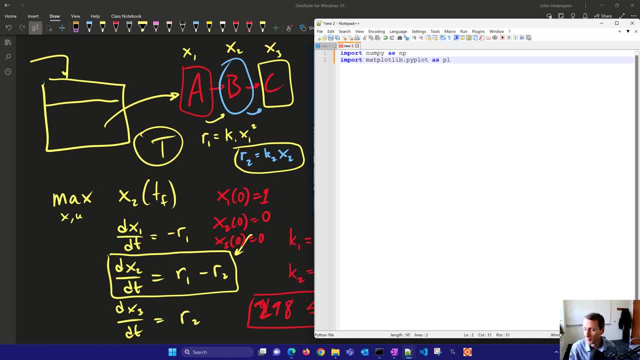 plot lib dot pi plot as PLT just to visualize the solution and then from gecko will import gecko. if you don't have gecko, just pip, install gecko. we'll create a new model. if you set remote equals false and it solves locally. we'll. 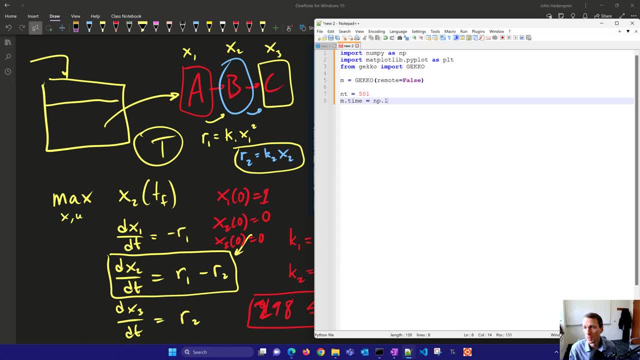 set up our time point. so I'm going to set up five hundred and one. so I'm going to set up five hundred and one of those, and then we'll linearly space them between zero and one, and then we'll have some variables as well: x1, x2 and x3. we'll start with an initial condition of 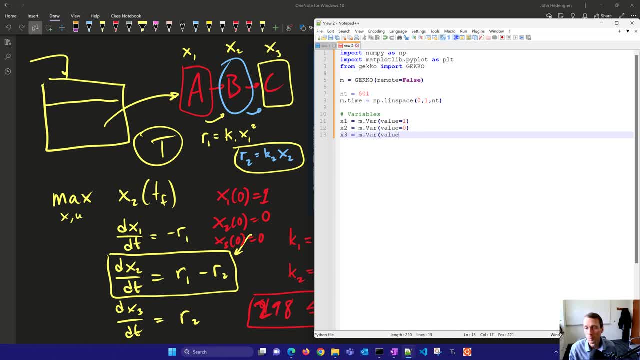 one, or x1 and x2. x3 will both be equal to zero. then we're gonna have our temperature and that's gonna be a manipulated variable and the value can go between 298 and 398. we'll give it an initial guess of 398 and then we'll have 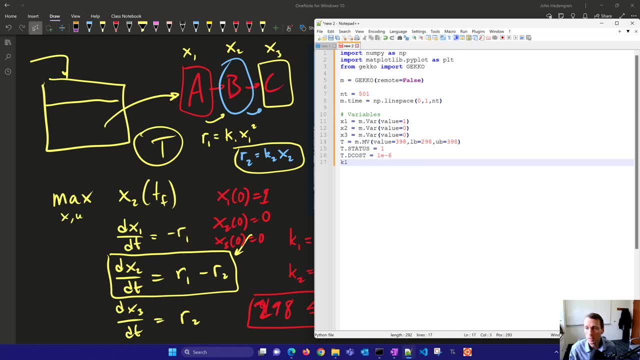 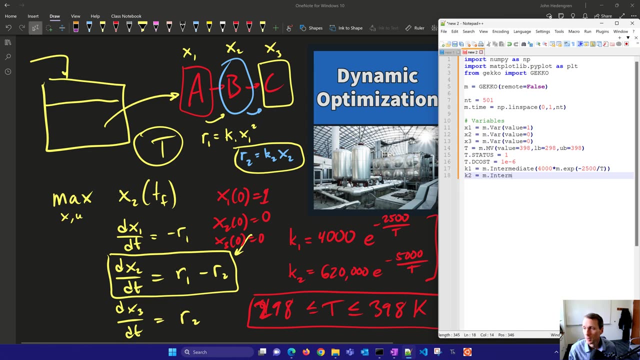 a value of 306, we'll turn it status on, meaning that the optimizer can adjust it. D cost put that a low value, so it just minimizes any chatter. now we're going to create some intermediates as well. these are going to be our k1 and k2 values. 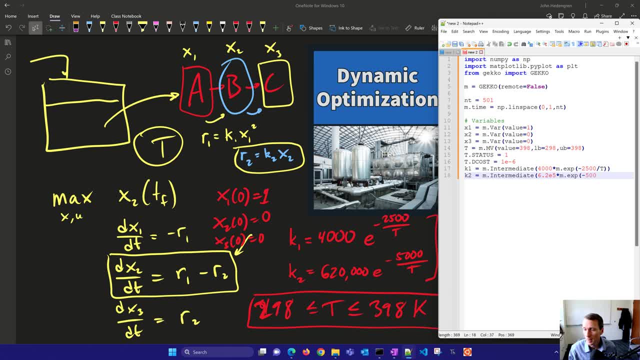 okay, that are right there. we've got our two intermediate values all right, and then we will have the final value here. this is going to la p. I'm going to set it equal to zeros with 501 points. the very last one's going to be equal to. 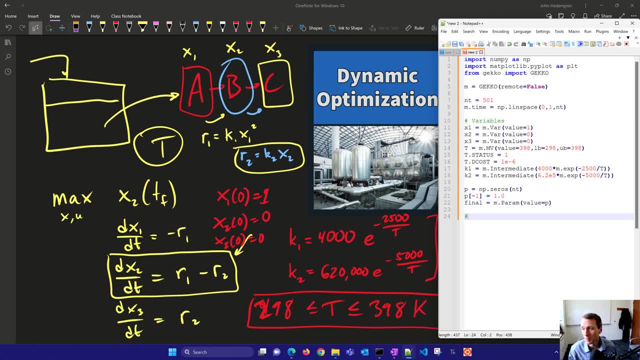 one. we'll set our final parameter basically with zeros everywhere except a one right at the end. that helps us maximize the amount of x2 at the very end. now we're going to create a reaction rate one and a reaction rate two. we'll set those up as intermediates because we use those later. 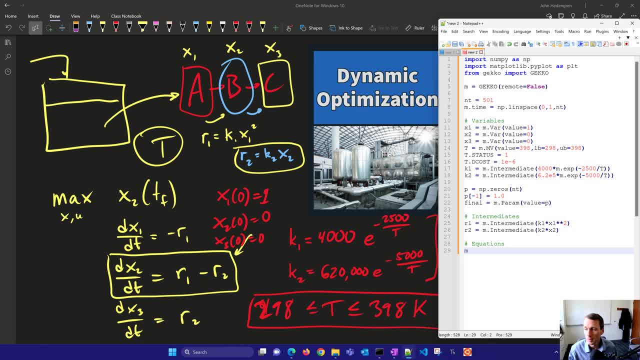 multiple places in the equations, and then in the equations we're going to set up the first one. this is just going to be the differential equation for a, and then we'll set up the differential equation for b. this is going to be our x2 and that's going to be reaction one minus reaction two. 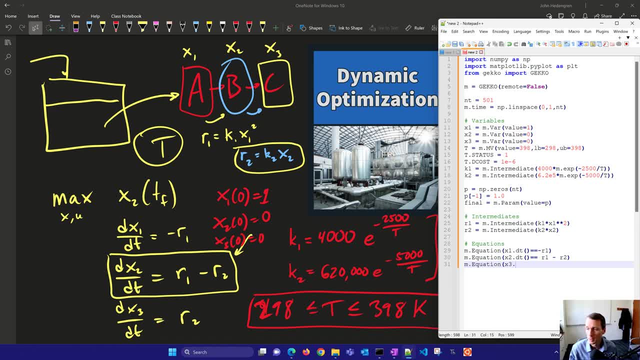 and then our third one, which is reaction. this is going to be the c, the undesirable product, and that equals reaction rate. two: now let's go ahead and create our objective function, and we're going to want to maximize the final x2 value. so we'll just 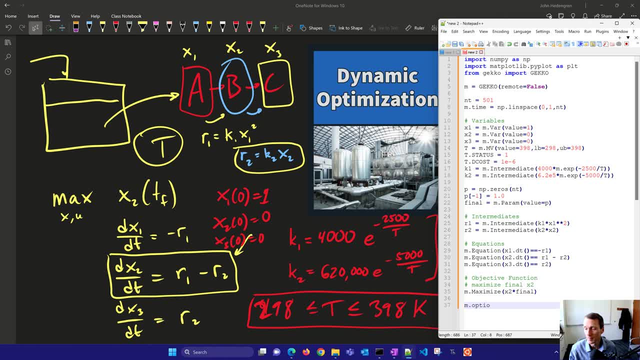 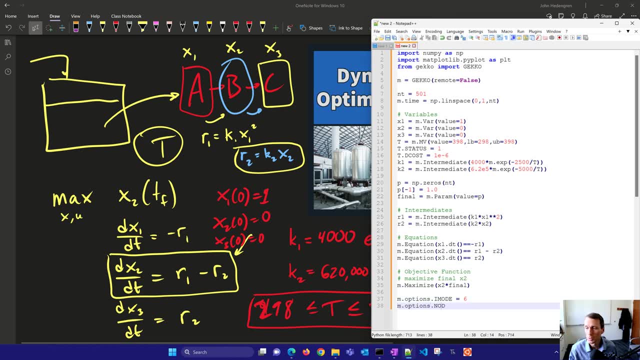 and we're going to maximize the final x2 value. so we'll just say: maximize x2 times final. so it's zero everywhere, except at the very end. then we're gonna set up I mode equals six- that's our dynamic optimization mode- and I'll set nodes equals three and then we'll solve it okay. so we're almost done. 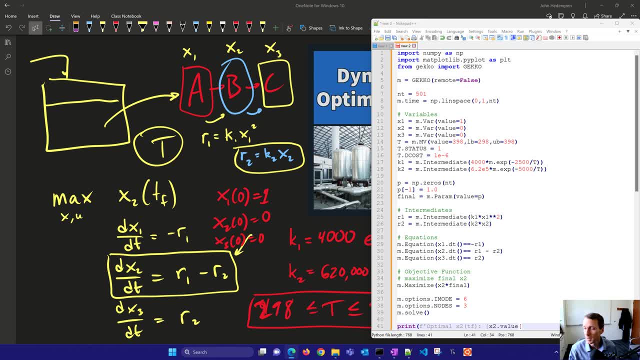 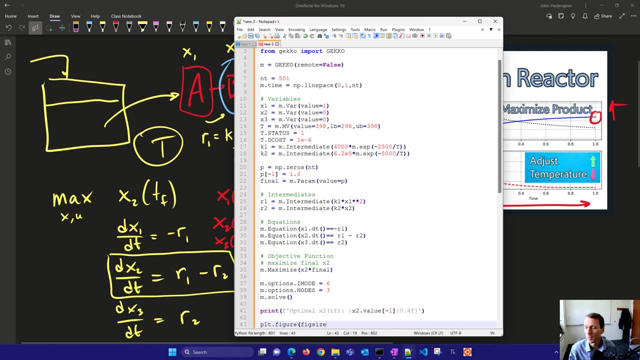 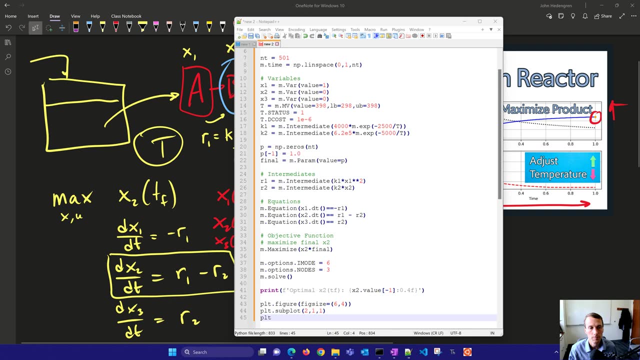 here. we're gonna just print out the solution. that's gonna be our final value with four decimal places, and then we'll also create a figure as well, with a couple subplots in there too. okay, we'll go ahead and run this just while it's generating this final plot. 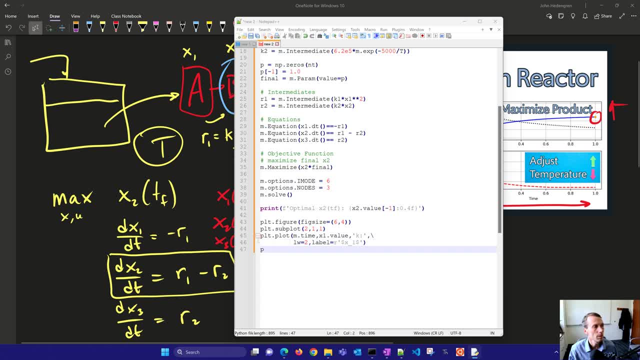 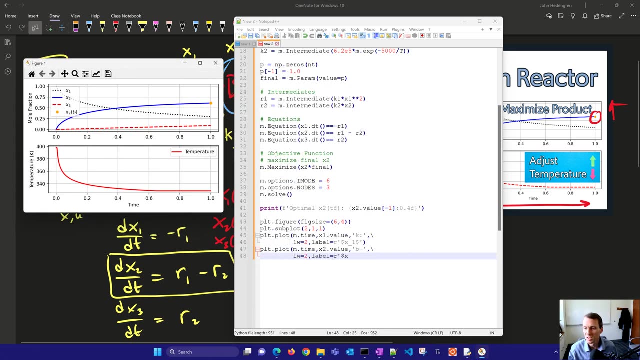 right here and we'll produce the final results. you me, okay, so let's just create this final plot, and here I'll just show the final plot just as we're generating it, just to see what we're doing. x1, x2, x3. you can see the rise of x3 here, the red line, the red dashed line. you can also see the. 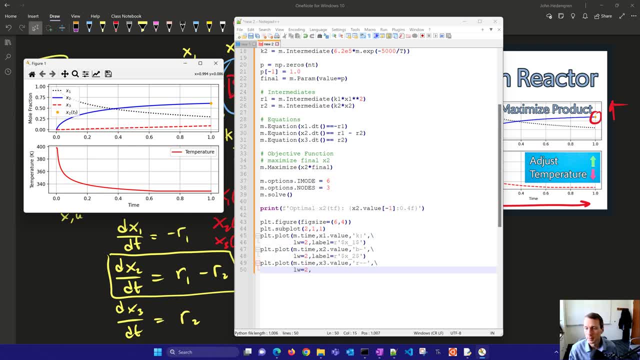 temperature profile as well. so we've got the three different concentrations of ABNC, pokc 1,, 2, and 3.. And then you could also see the orange dot there. That's our X2 at the very final time. That's the value that we're trying to maximize in the end. Now you can see here from: 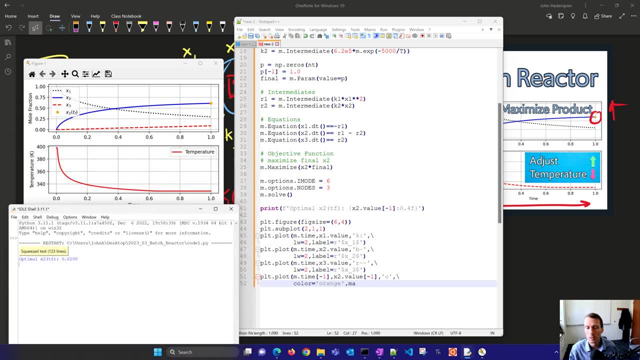 the solution that that is 0.6108.. And I just ran it with AP opt. It had 9,000 variables, 8,500 equations, 500 degrees of freedom. Those are my temperature values. I ran it with IP opt. 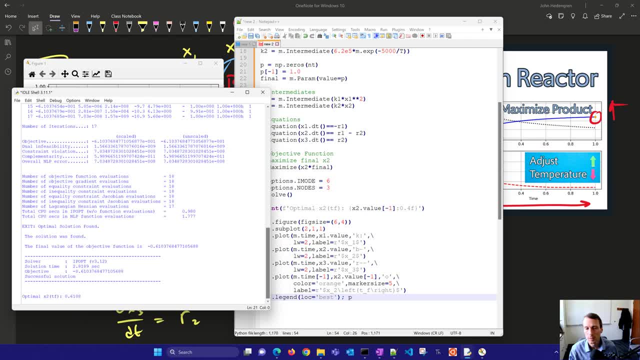 and you could see here the optimal objective was found And there you can see the optimal solution. Now, sometimes this is confusing. when you have a negative there, That just means that when we maximize, we multiply by negative one, because we have to convert it to a minimization. 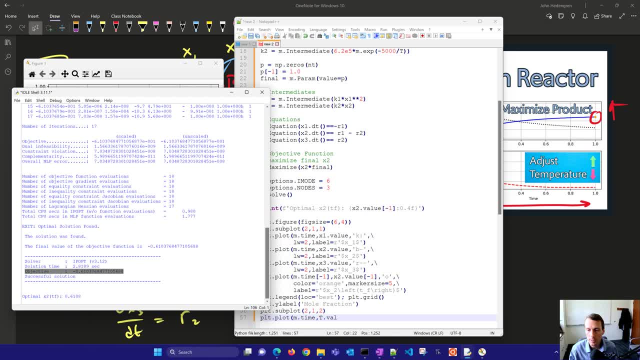 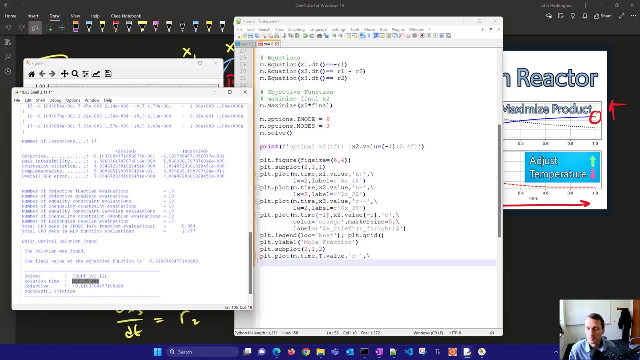 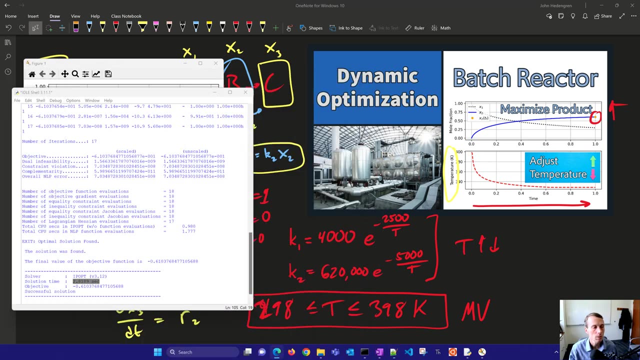 problem for IP opt And so that just has a negative value for the maximization. You can see it took about 2.8 seconds to solve this. Okay, So that is the batch solution If you need the source code for this. 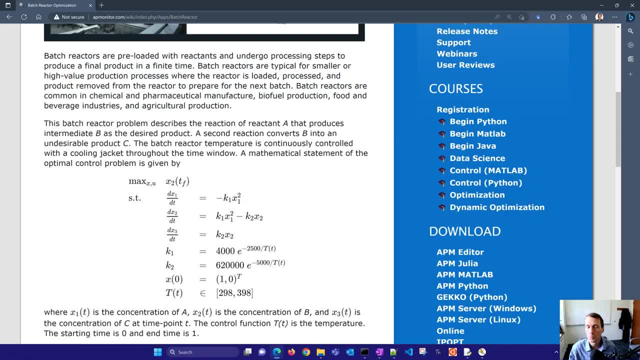 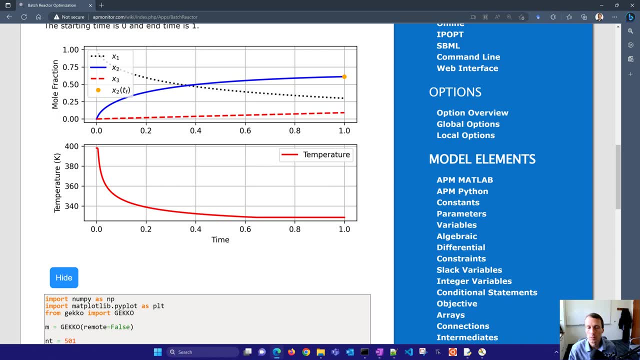 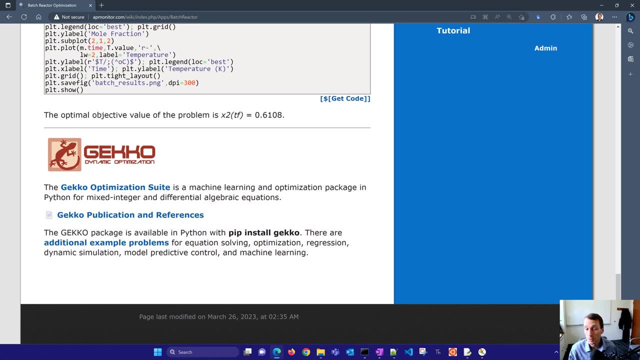 let me go ahead and just show that to you. It's here at this website, And down below you'll see a problem description along with the results and the solution. right here, the solution code. All right, This is solved with the Gecko optimization suite, If you'd like. 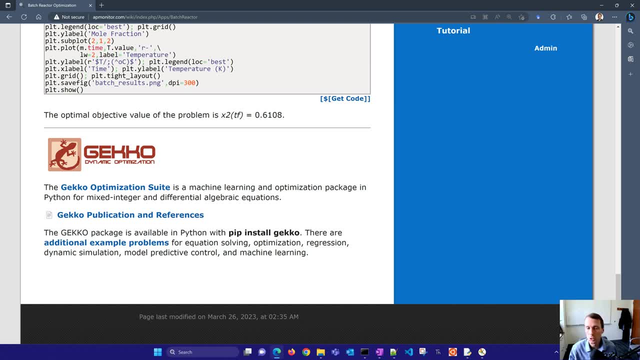 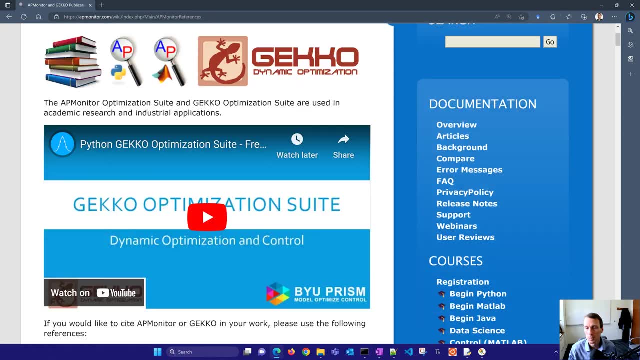 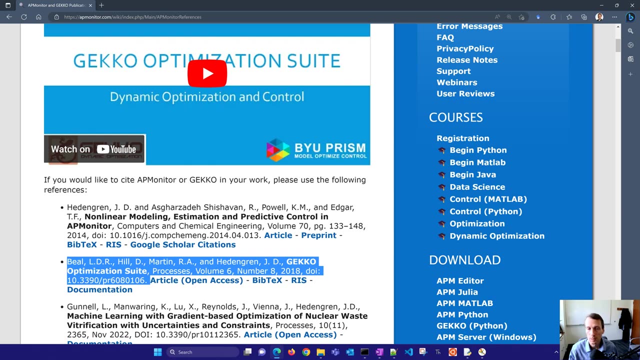 to see other applications of Gecko for mix, integer or optimal control problems or just optimization in general. select this link for Gecko references. You'll see the paper here. This is the Gecko paper where it gives a little bit more details about the algorithms. Also the AP monitor paper as well, And then a newer paper. 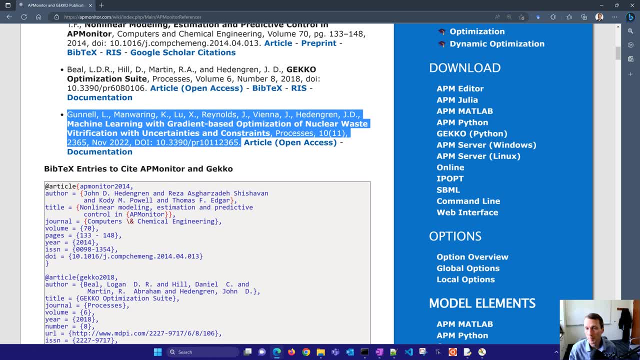 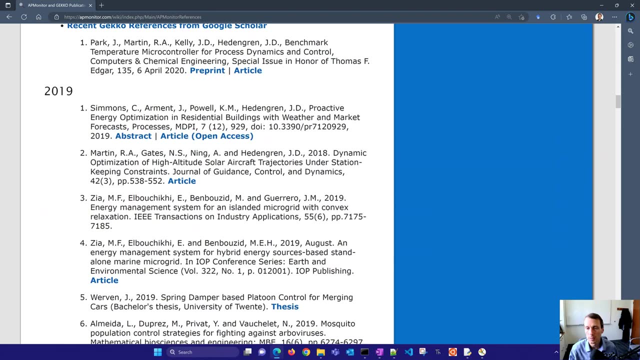 here where we've incorporated some of the machine learning packages like TensorFlow and SKLearn in with the Gecko package, So it gives a couple more methods there You can see here that you can use for modeling, And then there are some additional applications here You'll see a. 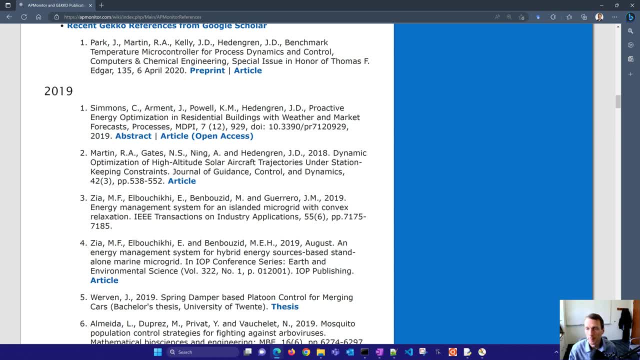 number of different applications with Gecko And you can see things like how to high altitude aircraft trajectories. Here you can see an energy management system for island microgrid. Here's a hybrid energy sources standalone marine microgrid. Okay, so a few microgrids. You also see things.